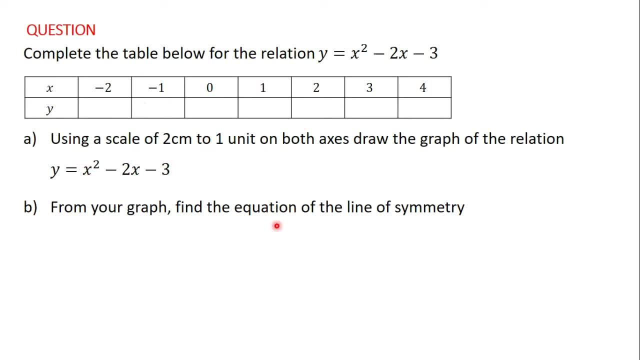 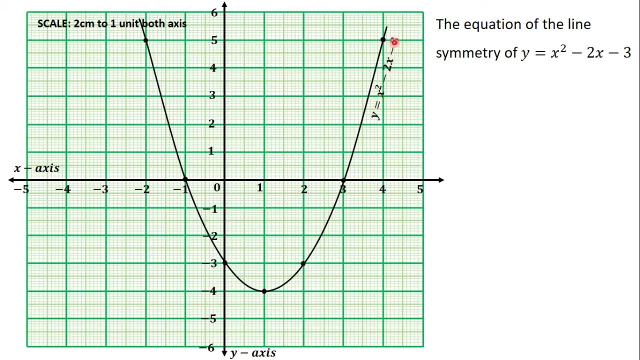 graph of this function. we will go straight to the last part of the question, that is, using the graph to find the equation of the line of symmetry. So this is the graph of the relation. y is equal to s squared minus 2x minus 3.. 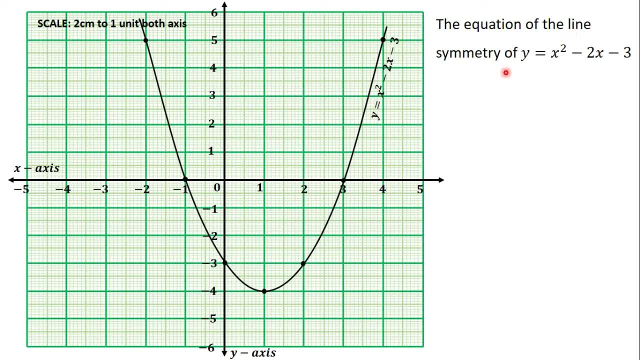 We are going to use the graph to find the equation of the line of symmetry. In the previous video, we learnt that to find the equation of the line of symmetry, the first thing you have to do is to locate the turning point of the curve. 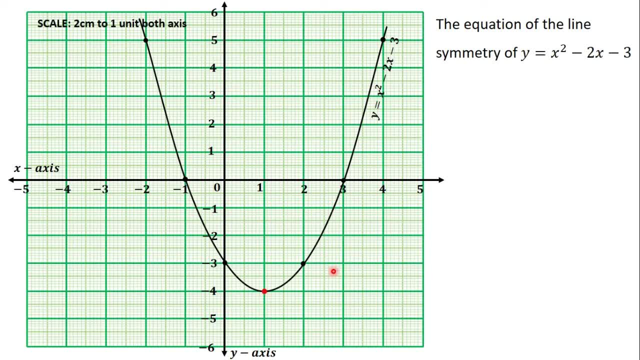 On our graph, we can see that this is the turning point. After you have located the turning point, you draw a vertical line through the turning point. This vertical line is known as the line of symmetry. So this is the line of symmetry of the curve. 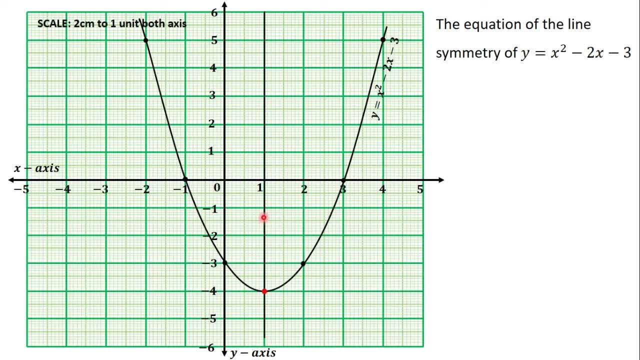 To find the equation of this line, you have to locate the point on the x-axis where the line meets the x-axis. As we can see, the line meets the x-axis at this point and at this point the x coordinate there is 1.. 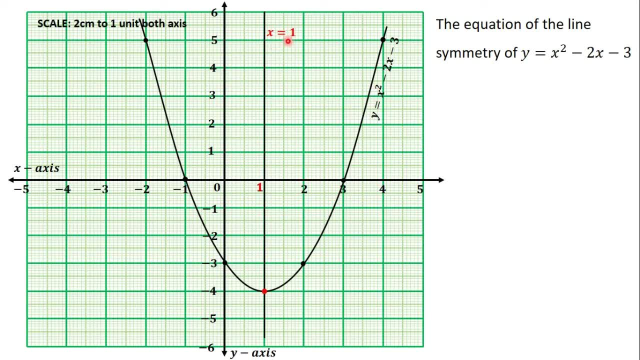 The equation of this line will be: x is equal to 1.. So from the graph we can see that the equation of the line of symmetry is: x is equal to 1.. It is very simple. Let's move on to the next question. 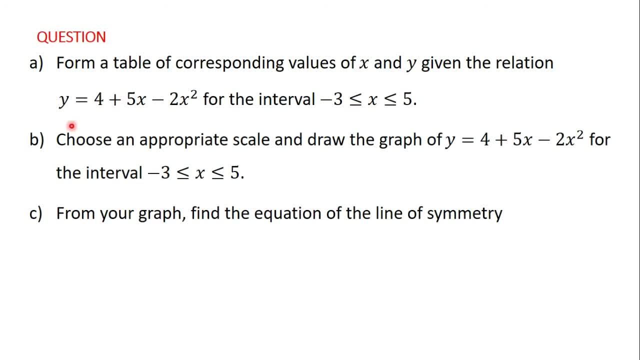 Form a table of corresponding values of x and y. for the relation y is equal to 4 plus 5x minus 2x squared. Then we will use the table of x and y values to draw the graph of the relation. y is equal to 4 plus 5x minus 2x squared. 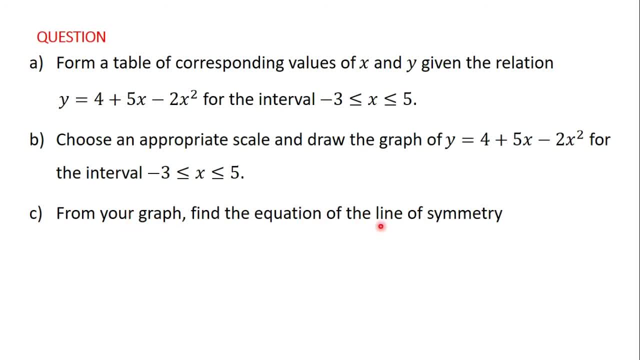 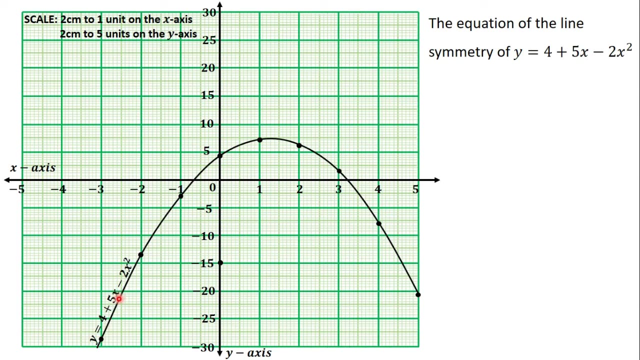 Then after that, we will use the graph to find the equation of the line of symmetry. Thank you, So let's go straight to the last part of the question, that is, finding the equation of the line of symmetry. This is the graph of the relation. y is equal to 4 plus 5x minus 2s squared. 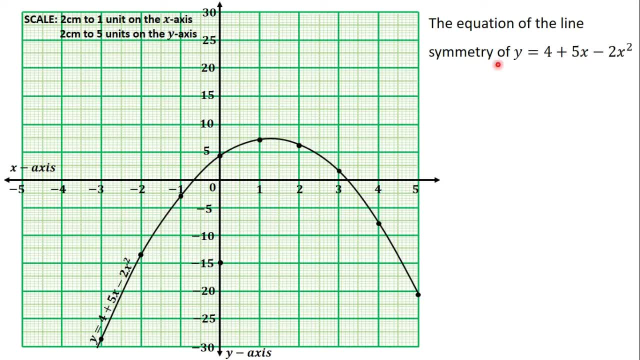 And we are going to use the graph to find the equation of the line of symmetry of y is equal to 4 plus 5x minus 2s squared. We have learnt that to find the equation of the line of symmetry, the first thing you have to do is to locate the turning point of the curve. 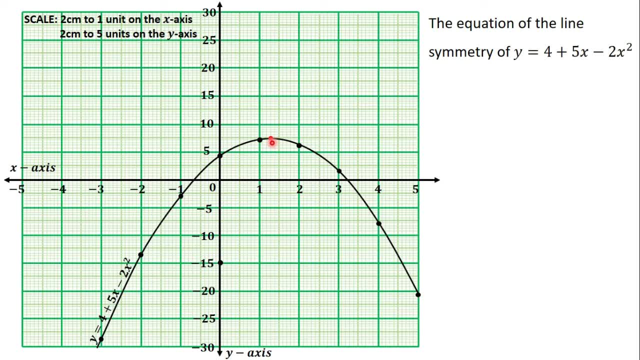 So on this graph, the turning point of the curve is at this point. After you have located the turning point, you draw a vertical line through it. This vertical line is known as the line of symmetry of the curve. So this is the line of symmetry. 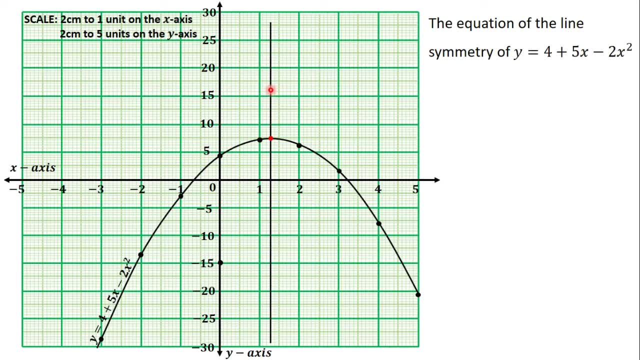 We want to find the equation of this line. To find the equation of this line, you go to the x-axis And you look for the point where the line meets the x-axis. As you can see, the line meets the x-axis at this point. 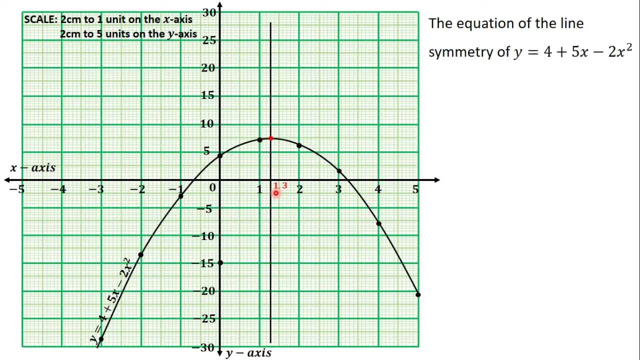 And at this point the x coordinate there on my graph sheet is 1.3.. So it means that the line meets the x-axis at the point 1.3.. The equation of this line will be: x is equal to 1.3.. 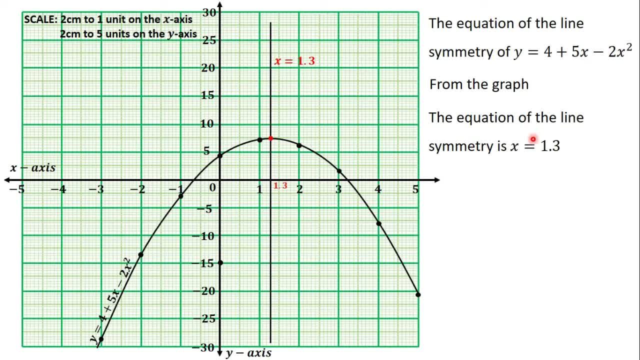 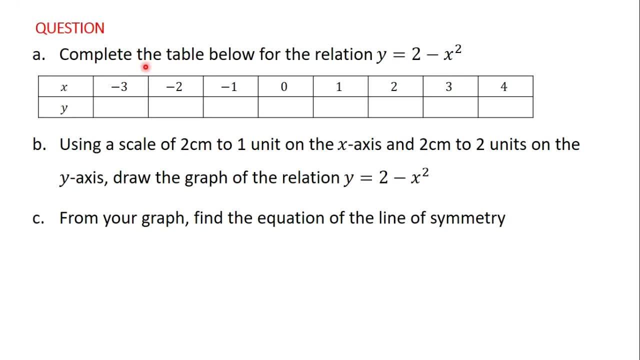 So from the graph, the equation of the line of symmetry is: x is equal to 1.3.. Let's move on to the next question. Complete the table below, for the relation y is equal to 2 minus s squared. Then after that we will used the values in the table to draw the graph. 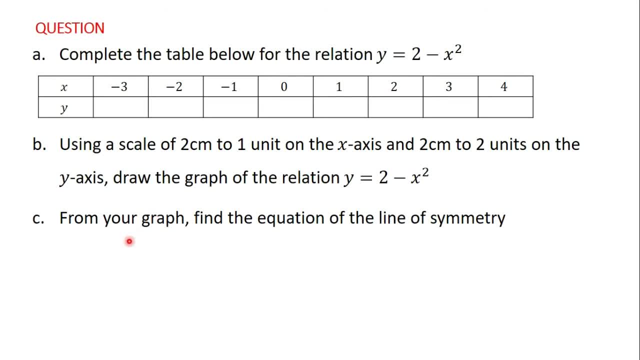 of the relation y is equal to 2 minus s squared, Then we are being told that from the graph we should find the equation of the line of symmetry. So let's learn how to use the graph- y is equal to two minus s squared- to find the equation of the line of. 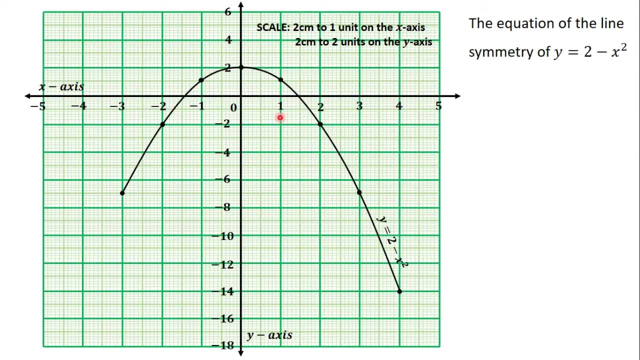 symmetry. this is the graph of the relation. y is equal to two minus s squared. we are going to use the graph to find the equation of the line of symmetry. as we have learnt to find the equation of the line of symmetry, the first thing we have to do is to locate the turning point of the curve on this. 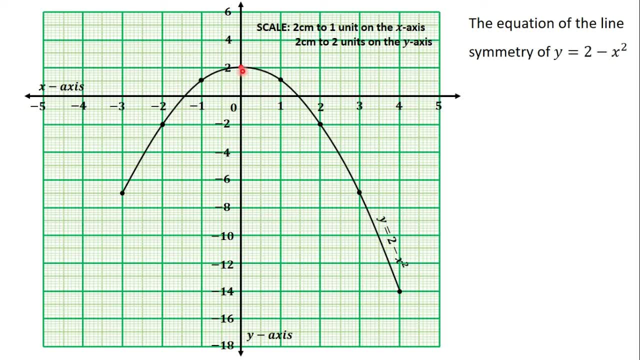 graph the turning point of the curve is at this point. after you have located a turning point, you draw a vertical line through the turning point. but you can see something very interesting on this graph: the turning point occurs on the y axis, so the vertical line through the turning point is the y axis. so on this, 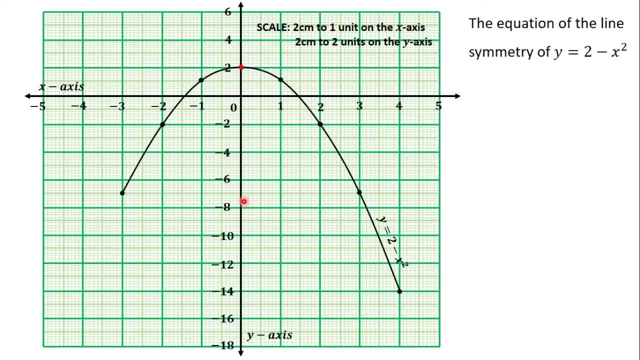 graph. the line of symmetry is the y axis. as we can see, the y axis meets the x axis at the origin, and at the origin, the x coordinate there is zero. so the equation of the y axis, that is the vertical line that passes through the turning point on, 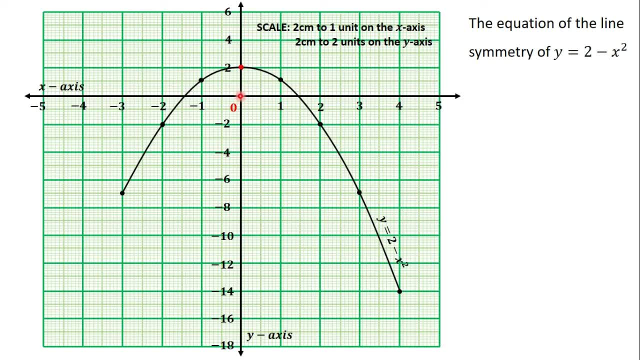 this curve is: x is equal to zero, because the y axis passes through zero on the x axis. so the equation of the y axis is: x is equal to zero and on our graph here the y axis is the line of symmetry. so on the graph the line of symmetry is the y axis. 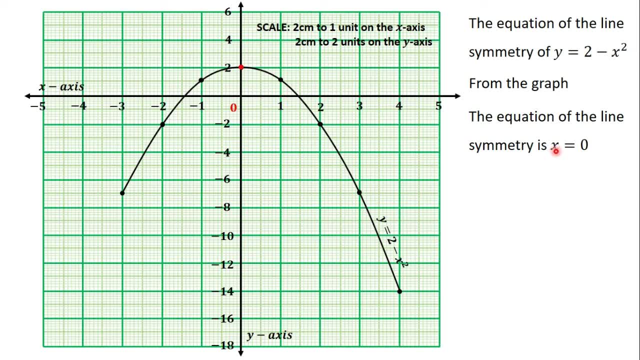 and the equation of the y axis is line x is equal to zero. so to find the equation of the line of symmetry you first locate the turning point. you draw a vertical line through the turning point. you will see that that vertical line will pass through a coordinate on the x axis. the equation of 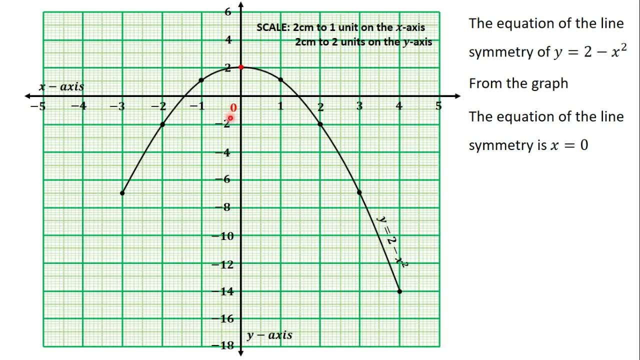 the line of symmetry is x is equal to that coordinate. on this graph, the line that passes through the turning point is the y axis and, as you can see, the y axis passes through the point zero on the x axis. so the equation of the y axis is x. 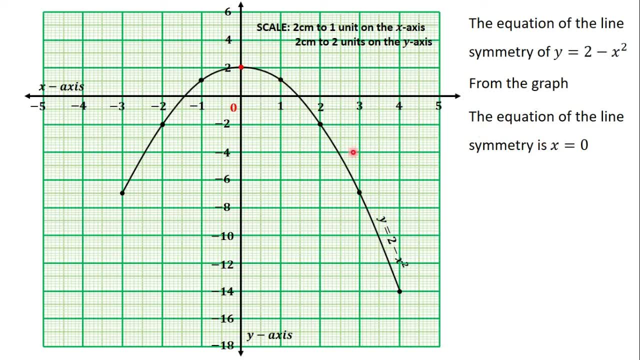 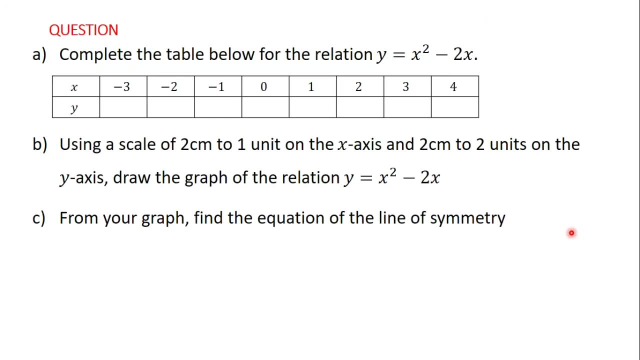 is equal to zero. so on this graph, the equation of the line of symmetry is: x is equal to zero. Let's look at the last question. Complete the table below, for the relation y is equal to s squared minus 2x. Then, using the values in the table, draw the graph of the relation y is equal to s squared. 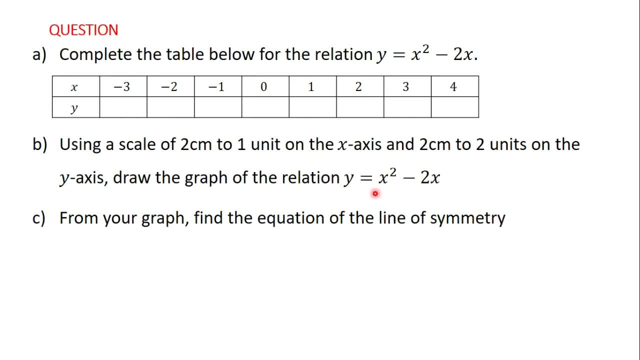 minus 2x. Then after that we will use the graph of the relation y is equal to s squared minus 2x to find the equation of the line of symmetry. So let's learn how to use the graph of the relation y is equal to s squared minus 2x. 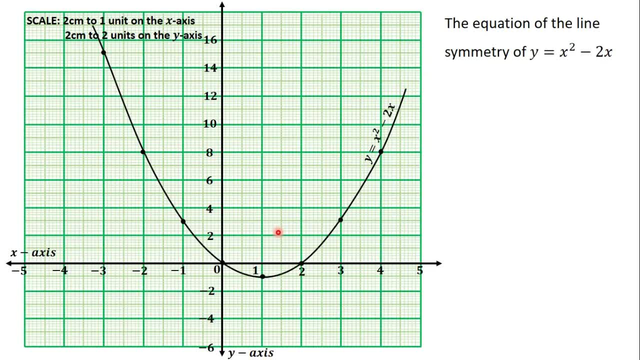 to find the equation of the line of symmetry. This is the graph of the relation. y is equal to s squared minus 2x, And using this graph we are going to find the equation of the line of symmetry. We have learnt that to find the equation of the line of symmetry, the first thing you